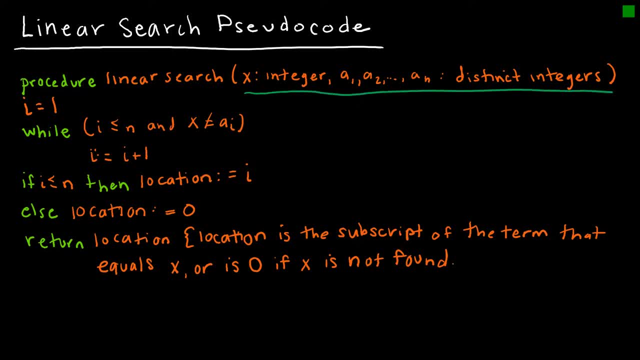 what values are the inputs? So the inputs are x and we're looking at the integers: a sub 1, sub 2, etc. all the way through a sub n, such that they are distinct integers, so no repeats. and then we're saying here let's start at the first value of the 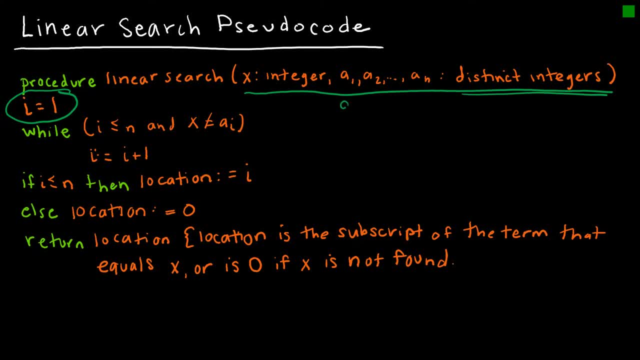 sequence, because a i equals 1 means a sub i equals a sub 1. that means we're starting right here. then we're telling the computer the process. so while i is less than or equal to n- remember what's n- that's the total number of numbers we have. so while there are still integers to look at, 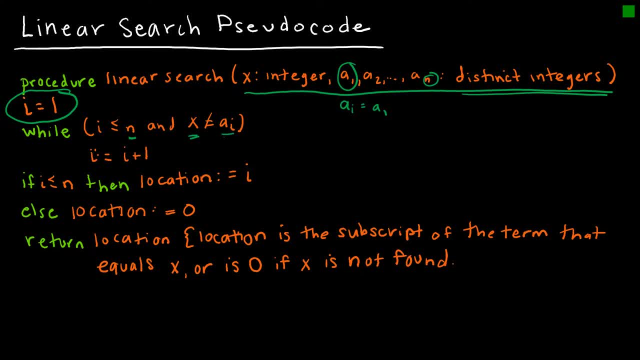 and x, our desired value is not equal to the value that we're checking, then we're going to go on to the next value in the sequence. so if a sub 1 isn't our x value we're looking for, then we're going to go on to a sub 1 plus 1, which, of course, is a sub 2.. 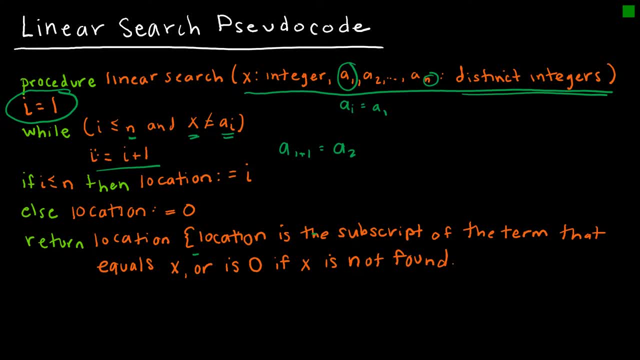 So then we say: if i- i being the subscript- is less than or equal to n, then the location is i, otherwise the location is 0.. So what does all that mean? That means it's a 0, if we haven't found the value that we're looking for. 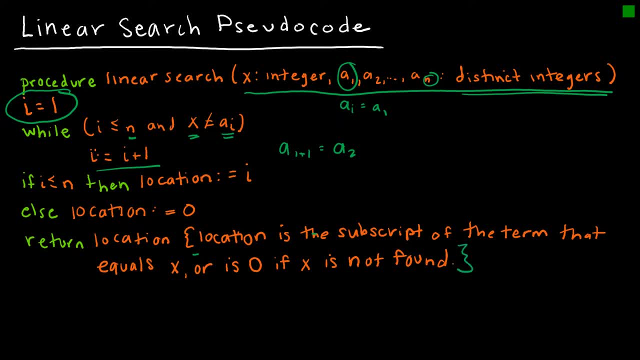 What's the return? And again, there should be a bracket on the edge of that, I apologize. The return is the location and the location is i, such that i gives us the location of our value of x. So location is the subscript, which is i, of the term that equals x or 0, if it is not found. 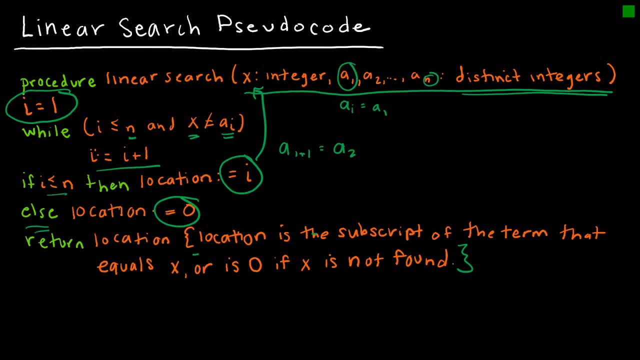 So that's where that else comes in. So if i is less than or equal to n, then it's a 0 if we haven't found the value of x. So if i is less than or equal to n, then the location is i. otherwise the location is 0, meaning it was not found. 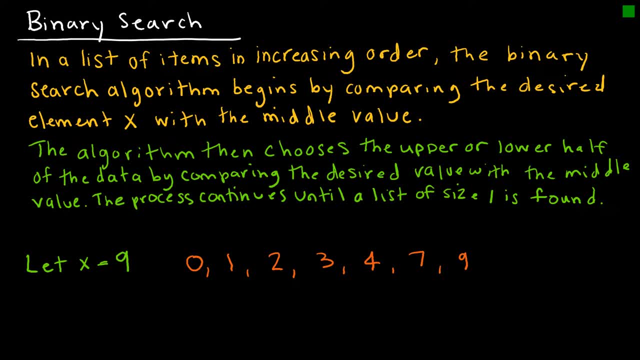 So now let's look at the binary search algorithm, which is another search algorithm, And the only difference here- or the biggest difference here- is that the list of items must be in increasing order. So it's possible that you might have to do some sort of sorting algorithm first if you have data that's not in the correct order. 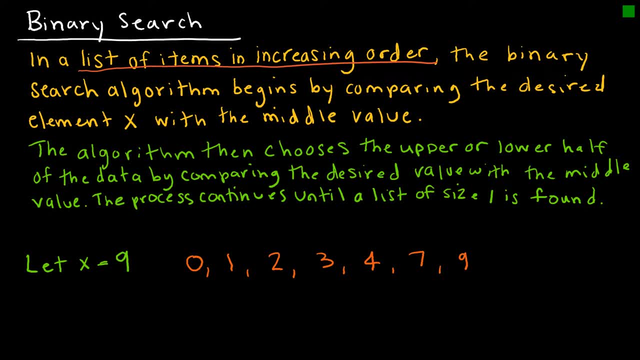 and then use the binary search algorithm, And this one basically begins by comparing the desired element x with the middle value. So, specifically, what it does is it looks at the fact that this is a1,, a2,, a3, etc. And it says: okay, the left endpoint is a1 and the right endpoint is a7. 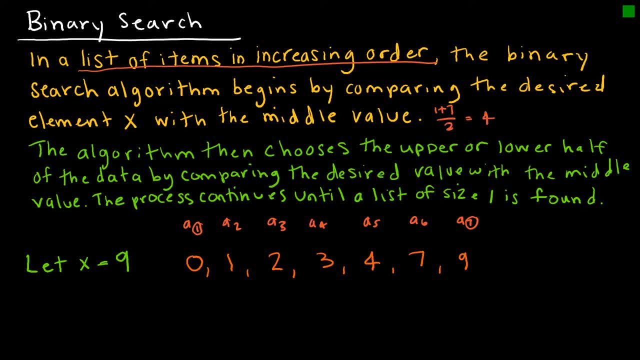 So we're going to take 1 plus 7 and divide it by 2 to get 4.. So let's look at what's happening at a4.. At a4, our value is 3.. So let's compare 3 to 9.. 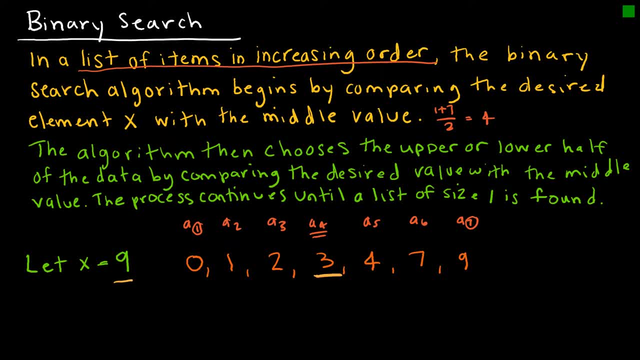 Well, 9 is greater than 3.. So because it's greater than 3, our algorithm says: okay, let's use this as the left endpoint and still keep this as the right endpoint. So essentially it's saying let's get rid of this data. 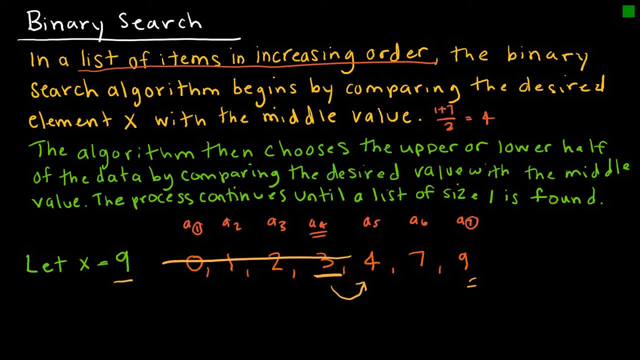 If our value was less than 3, then we would have included all of this to determine the left and right endpoints. So it would be a1 and a4 and continue from there. But because it was to the right now, I'm left with a5, a6, a7. 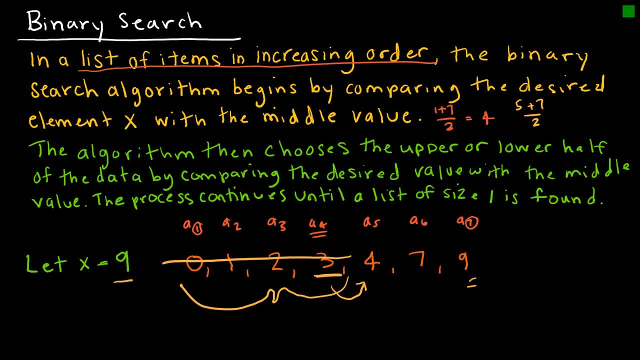 So I'm going to take 5 plus 7 and I'm going to divide it by 2, which of course gives me 6.. And that tells me to now compare the value at a6, which is 7, to the value that I'm looking for, the desired value of 9.. 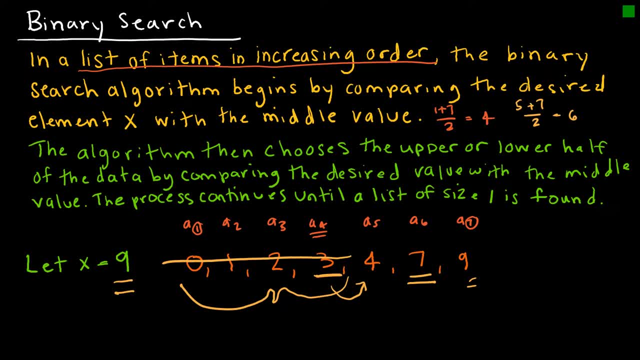 And 9 is greater. So again, this tells us: if it's greater than this, then this is the left endpoint. So these go away, And so the left endpoint is 7 and the right endpoint is 7.. So, basically, we now found a list of size 1, which is what we wanted. 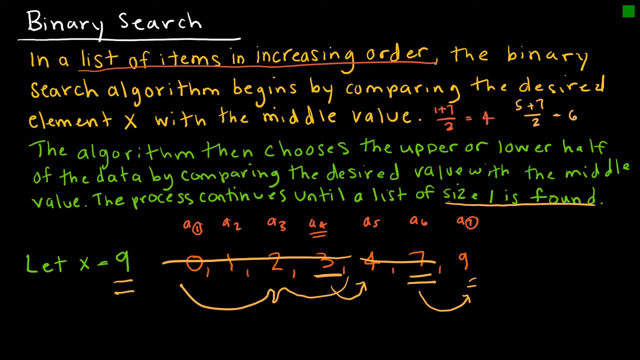 And what my output would be then is either 0,. if this answer wasn't 9,, then my output would be 0., But because the answer is 9,, the output is the least. So that's the location of the solution, which is in the 7th position. 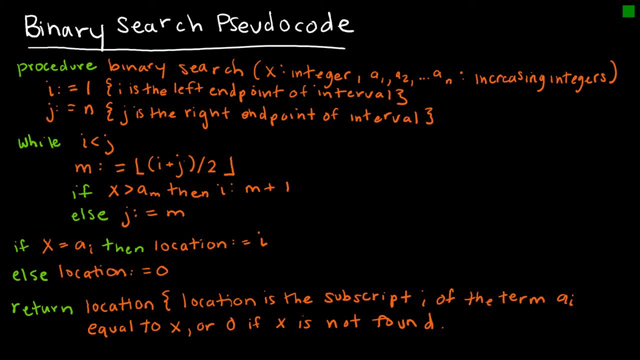 Let's take a look at the pseudocode for that binary search algorithm. Again, the procedure we're calling binary search, we're saying that we're using, we're finding x And we're trying to find x in a list of integers ordered from a1 through a9 that are increasing integers. 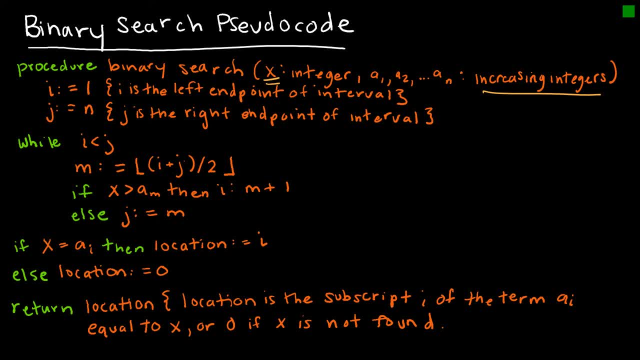 We're saying that i is going to represent the left endpoint of the interval and it's going to start at i, Or sorry, at 1, because 1 is when we start is the left endpoint. for sure. j is going to start at n and that's going to always be the right endpoint of our interval. 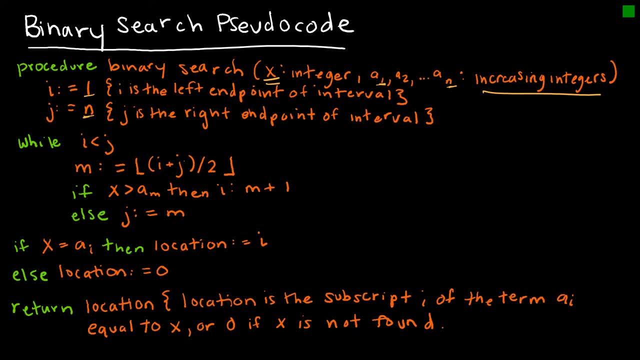 And then we're saying: while i is less than j, so while essentially we don't have a list of 1, we're going to take the floor function of i plus j divided by 2.. So we didn't have to end up doing the floor function in our last example, just because that's the way it worked out. 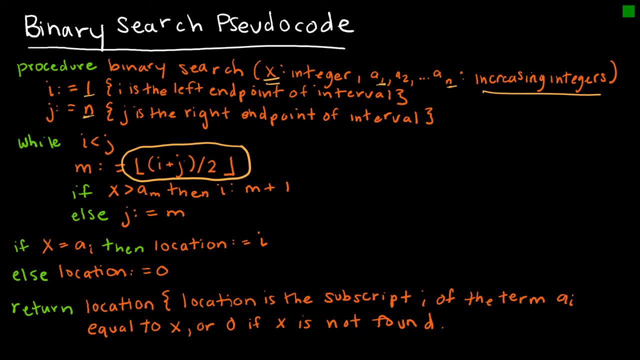 But if we had to we would have done the floor function rounded down to the nearest tall integer. We're basically taking the subscripts or the locations of the left and right endpoint and dividing by 2.. Then we're saying if x, our desired value, is greater than that middle value. 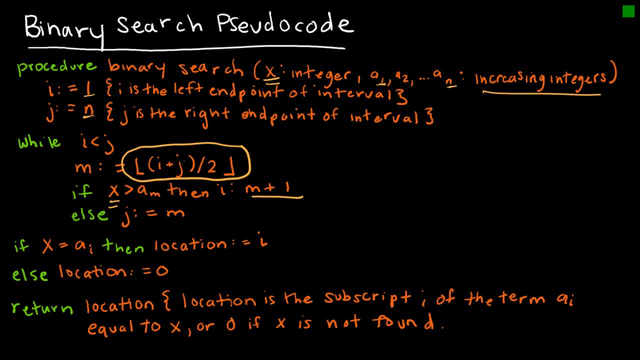 then my new left endpoint is 1 to the right of that, which is what we did. Otherwise, j, which is the left endpoint, is going to be that middle value that we used. So if x is equal to a sub i, then that is the location. 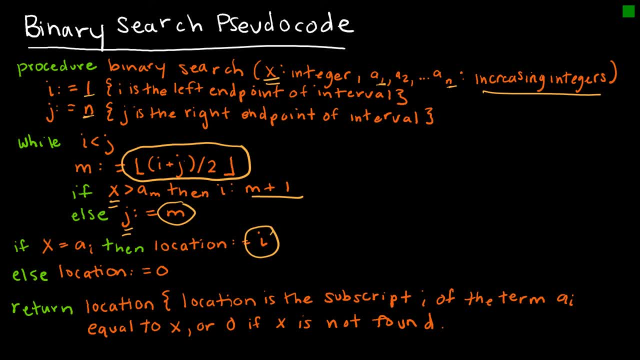 If I didn't find the desired value of x, then my location is 0. And then the return or the output is the location. And again all of this stuff- and I keep forgetting to put the second bracket on, but all of that stuff in the middle is basically just telling us, as a person, what the location is. 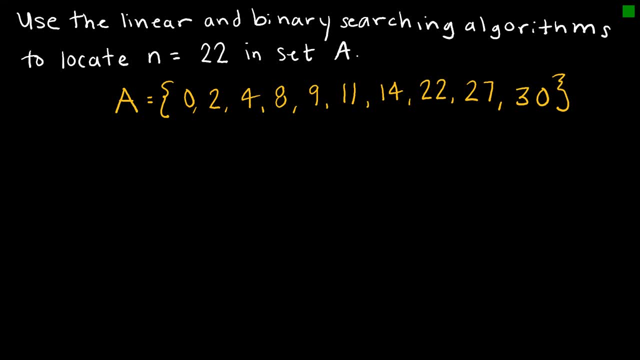 So here's a problem Practice for us. We're looking for the value of 22 in a set And here is the set. And notice: I was nice enough to put these in the correct order for you already, So if I were using the linear search algorithm, 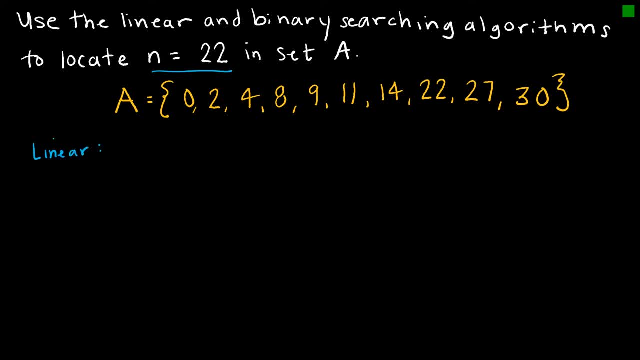 then I would look for- and again I should number these a1,, a2,, a3,, a4, etc. And I'm not going to cross them off as I did last time, because obviously I'm going to use them again when I do my binary search.